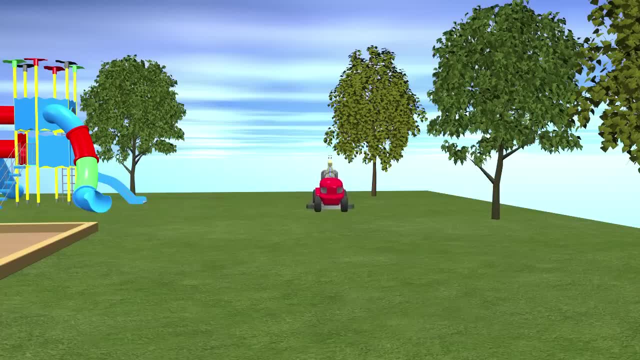 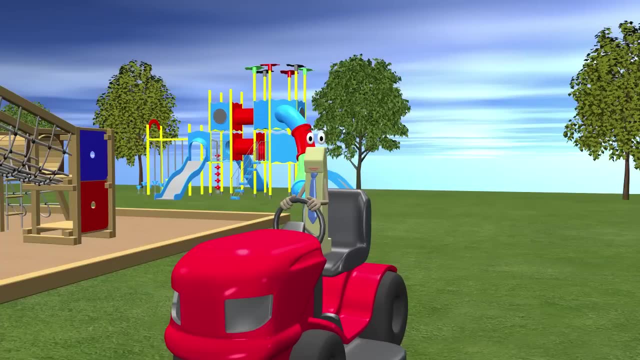 Hey kids, how are you guys doing today? Great, Hey, I recently got a job mowing lawns for this park. I started to earn some money, but I was wondering if you can help me learn about money, so I will know how much I am earning. 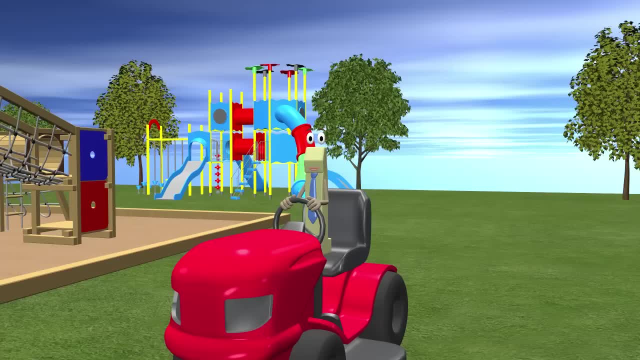 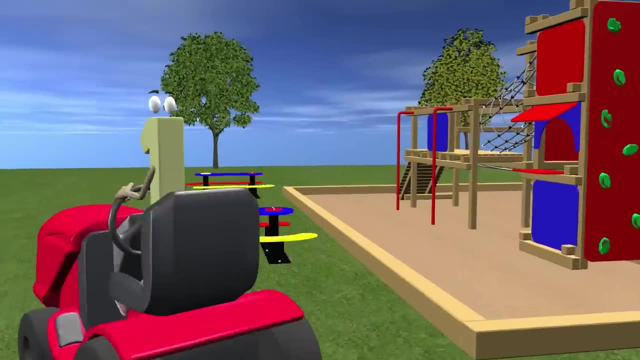 Can you guys help me with that? Thanks guys. Okay, let's go over to the table and look at some coins and see if we can make sense of it. Here on the table we have a golden diamond ring. On the right we have a big rock. 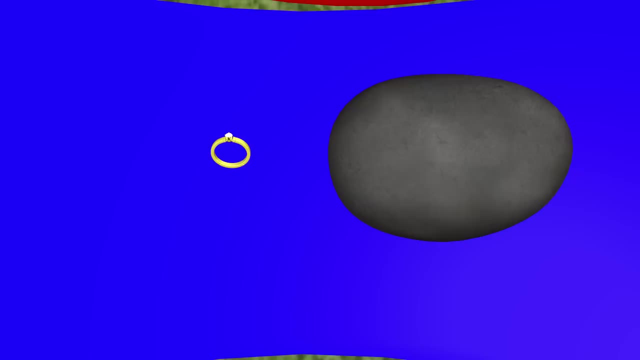 Which one of these objects is bigger: the diamond ring or the rock? Yeah, the rock is totally bigger. Now can you tell me which one of these objects is worth more money? I heard someone say the diamond ring is worth more money, but how The rock is so much bigger. 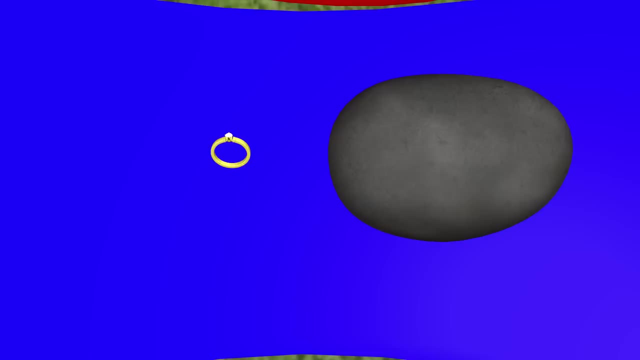 Yeah, the diamond ring is definitely worth more than the rock, though Even though the ring is smaller, it is still worth more than the rock. And did you notice? there is only one diamond ring and one rock, So even though there is only one of each, each of them has a different value. 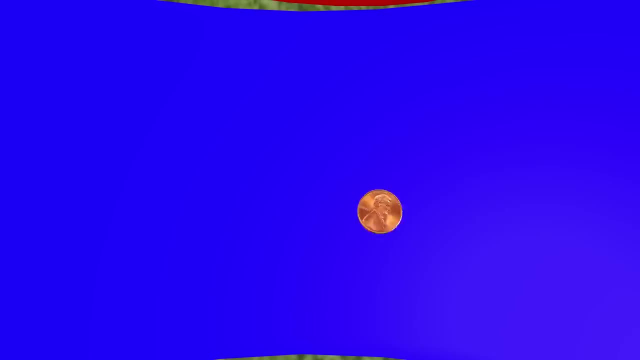 Let's look at some coins now and I will show you what I mean. This coin is called a penny. A penny is worth only one cent. The word cent is used when talking about coins. This is the cent symbol. Okay, let's use our tens blocks to compare the worth or value of this coin. 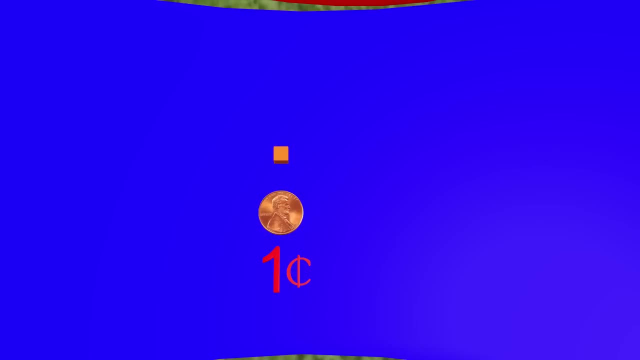 The penny is only worth one cent. as we see here, This next coin is called a nickel. A nickel is worth five cents. These five ones blocks represent the value of this nickel. So the penny is worth one cent and the nickel is worth five cents. 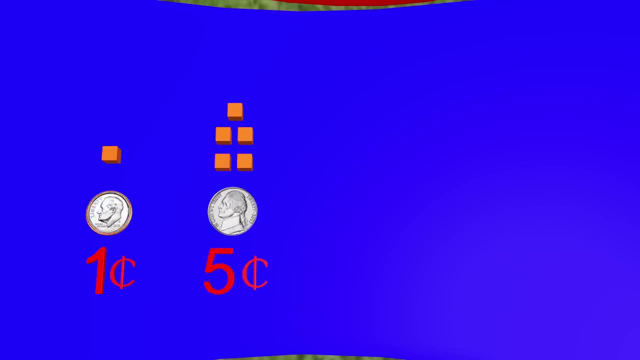 Our next coin is smaller than the nickel and the penny, But just as we learned with the ring and the rock, the size is not important. This coin is called a dime. A dime is worth ten cents. We can see this with one of our tens blocks. 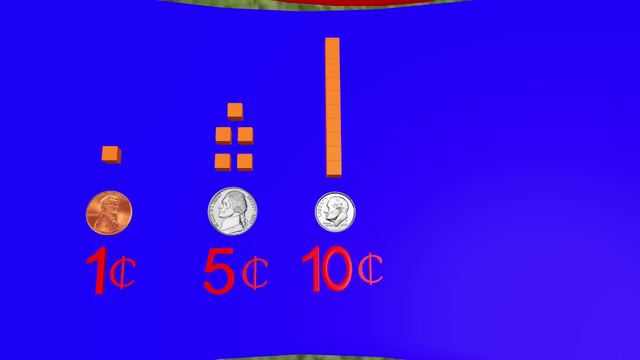 This tens block has ten blocks in it, so it represents the dime. So the penny is worth one cent, the nickel is worth five cents and the dime is worth ten cents. Our last coin is called a quarter. A quarter is worth twenty-five cents. 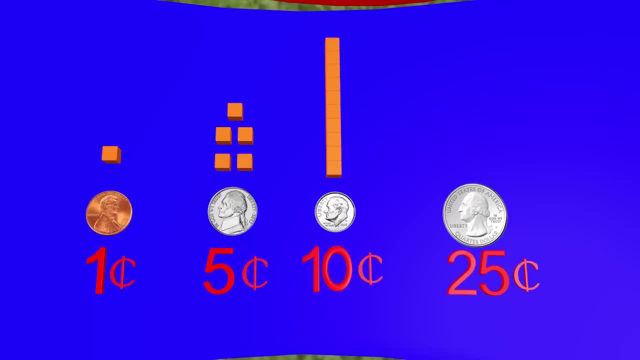 To show twenty-five cents with our blocks, we would need twenty-five blocks, right? So to get twenty-five blocks, we need two tens blocks and five ones blocks. This set of tens blocks represents a quarter. So we have our penny that is worth one cent, our nickel that is worth five cents. 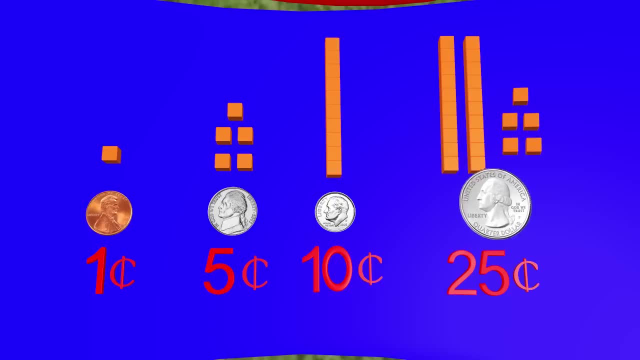 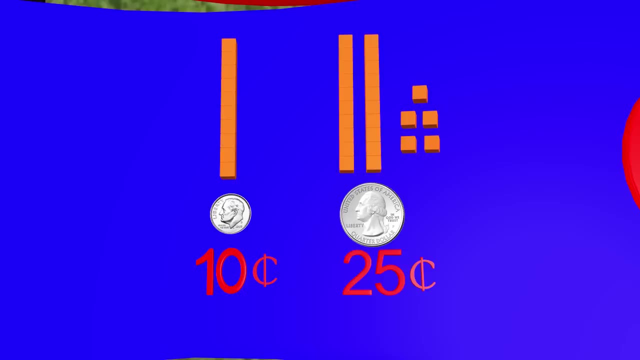 our dime that is worth ten cents and last of all, our quarter that is worth twenty-five cents. Okay, can you tell me which coin is worth more, the dime or the quarter? The quarter is worth more. We can see that the dime is worth ten of these blocks. 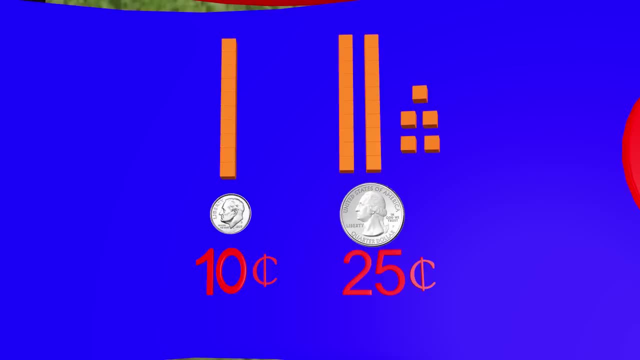 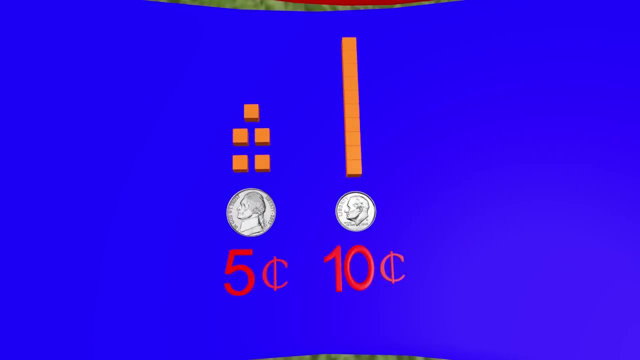 and the quarter is worth twenty-five of these blocks. A quarter is worth more than a dime. Which coin is worth more here, the nickel or the dime? The dime is worth more. Good job. The dime is worth ten cents And the nickel is worth five cents. 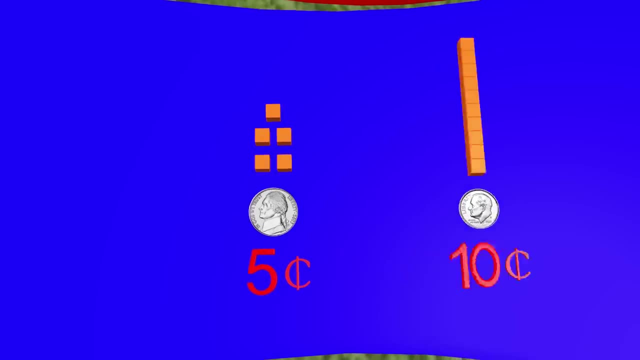 Ten is more than five. Let's look at one more. Here we have the penny and the nickel. Which coin is worth more? Good job, The nickel is worth more than the penny. The penny is worth one cent And the nickel is worth five cents. 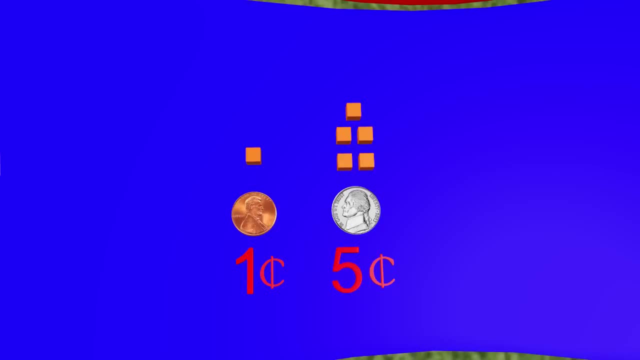 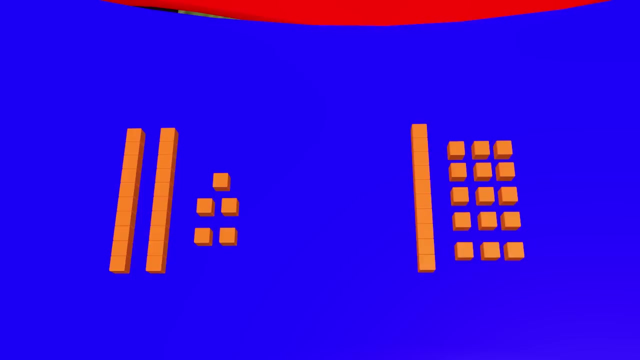 Since each of these coins has a different value, there are many ways to add these up. For example, I am getting paid twenty-five cents to mow this lawn. Let's look at some ways I can get paid twenty-five cents. Here are a couple of ways we can get twenty-five cents. 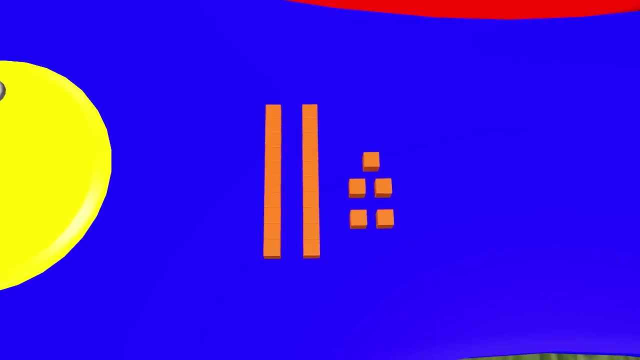 We are using the blocks to help us. Here we have two tens blocks and five ones. These two tens blocks can each be dimes, since they both represent ten. The five ones can represent a nickel, since a nickel is worth five cents.